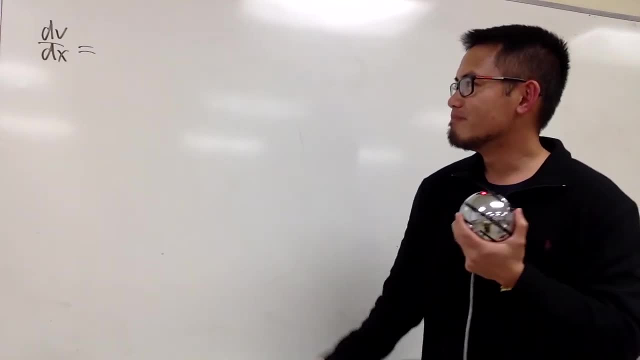 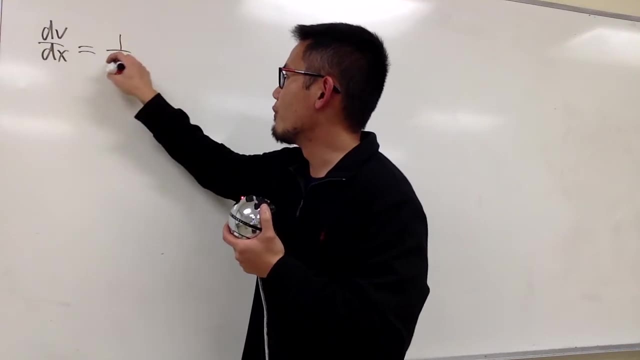 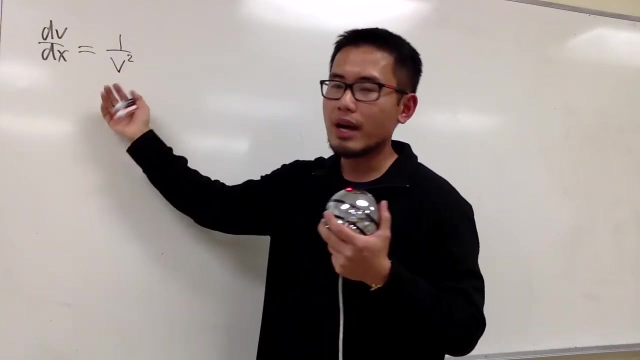 And just make it something easy. okay, And if you have seen my previous video, this is what I did. I start with dVdx and I'll make this equal to 1 over V squared. So, as you can see, this is solvable by separating the variable right. 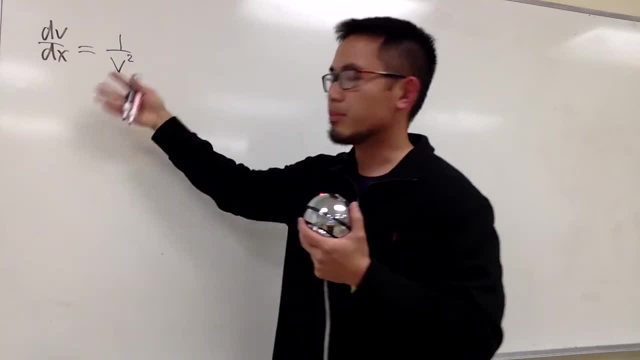 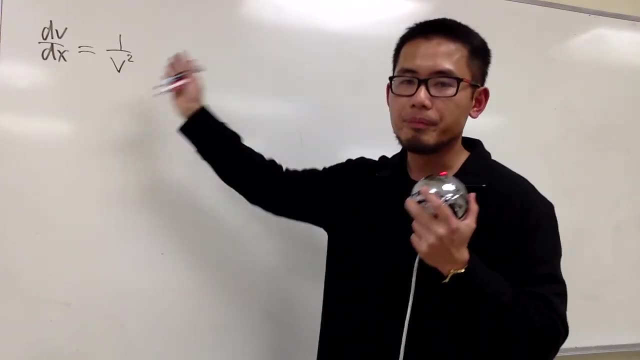 I can just multiply V squared on both sides and multiply the dx on both sides, so we can just integrate both sides. That's pretty much it. So, that's pretty much. you start with an easy enough differential equation in terms of V. 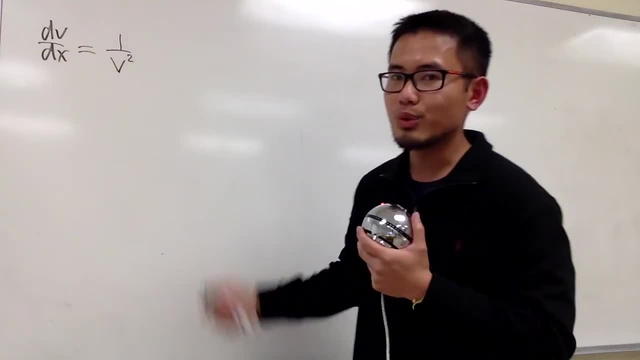 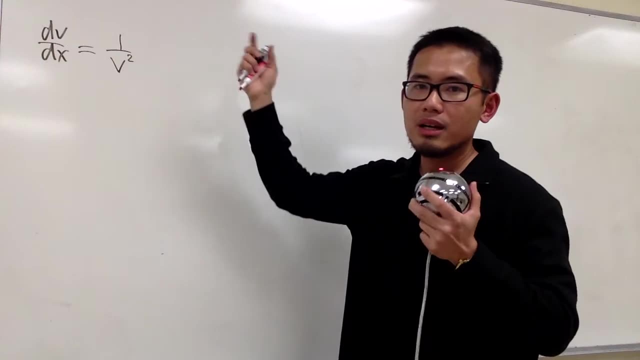 And if you want You can put down some x right here on the right-hand side as well, And just you have to make sure this right here is easy enough to solve, Maybe by separating the variable, or maybe by the first-order linear differential equation, the integrating factor, things like that. 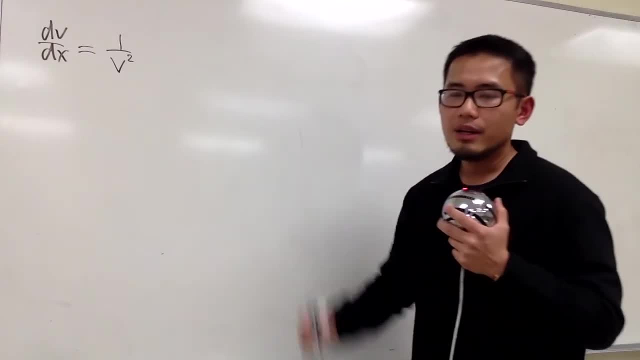 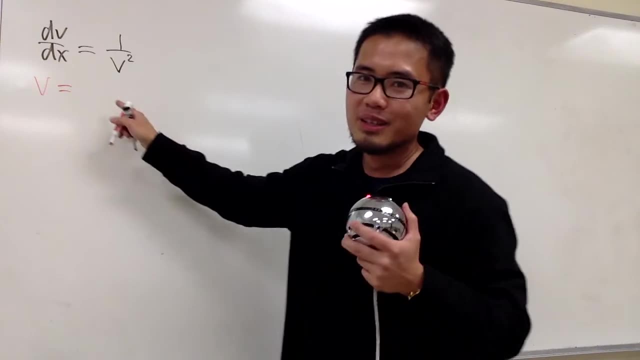 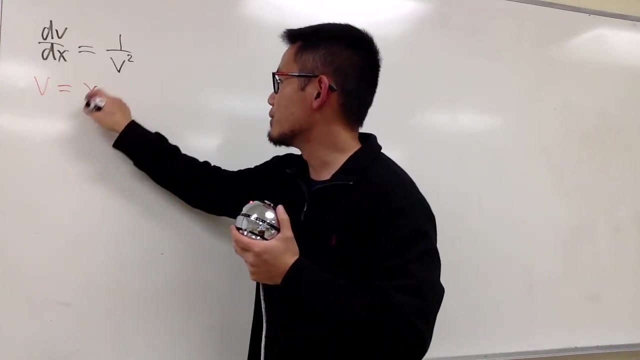 Okay, Alright, now this is V and you are going to decide whatever you want, alright. So in my previous video I left: V equals to whatever you want in terms of x and y. Of course, keep it reasonable And I chose to do x to the 3rd power plus y to the 3rd power. 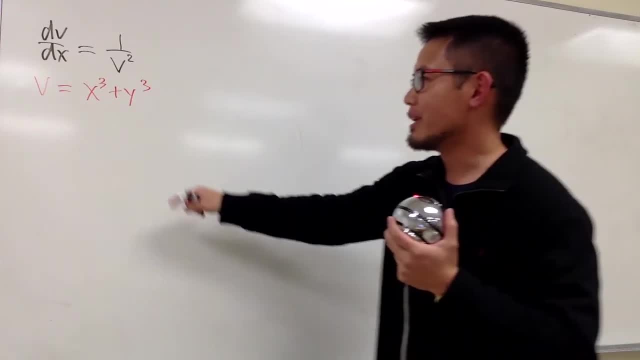 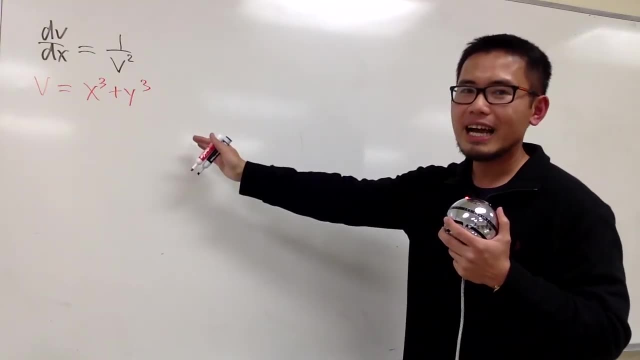 And seriously, right here you can do whatever you want. You can even do sine of x times y inside like this. But this is it I left. V equals to x to the 3rd power plus y to the 3rd power. 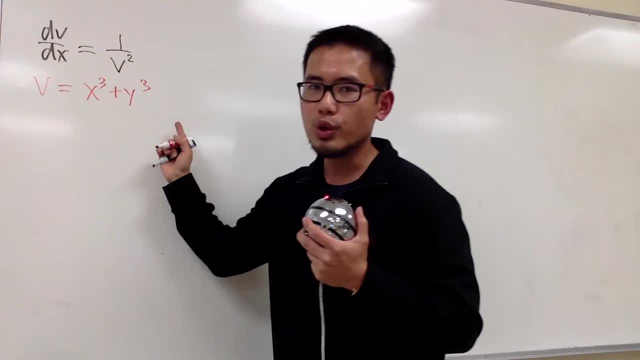 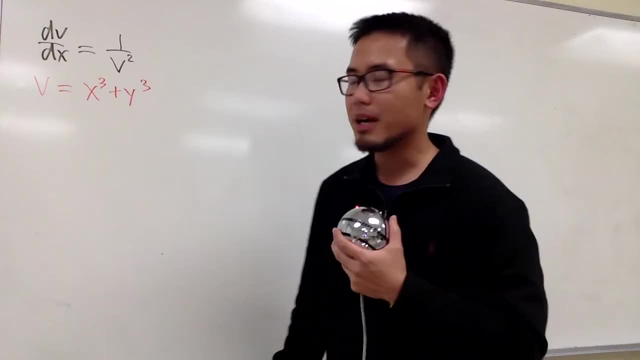 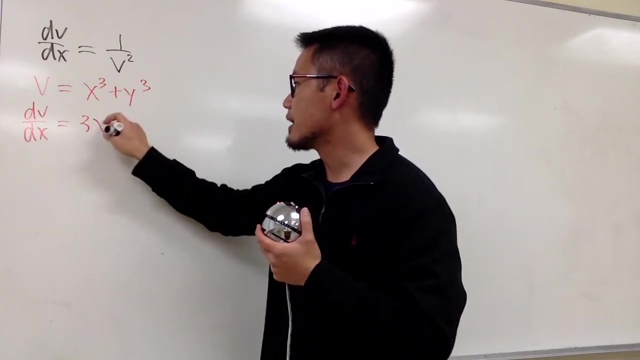 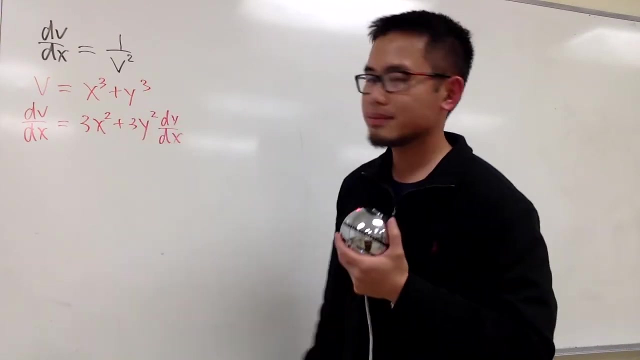 And then next is that I will look at this differential equation and differentiate both sides And keep in mind V is a function of x, Y is also a function of x. Keep this in mind. Okay, so on the left-hand side, I differentiate that I get dV dx and this will be 3x squared plus. this is going to give us 3y squared dy dx. 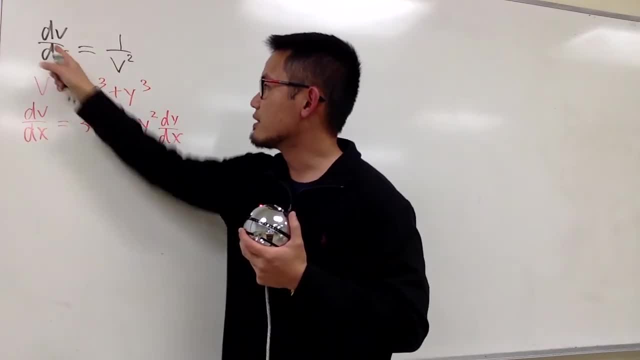 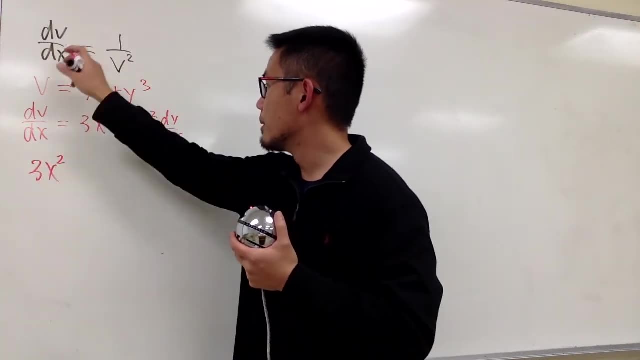 And you see, right away we have the dV dx, right. So now I can just put this to that and we will have 3x squared plus 3y squared dy dx, And this is equal to 3x squared dy dx. 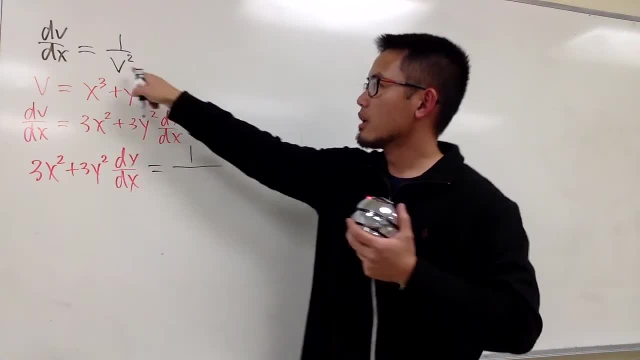 And this is equal to 3x. squared dy, dx, And this is equal to 1. over here I have the V squared right, But V. I set it to be x to the 3rd power plus y to the 3rd power. 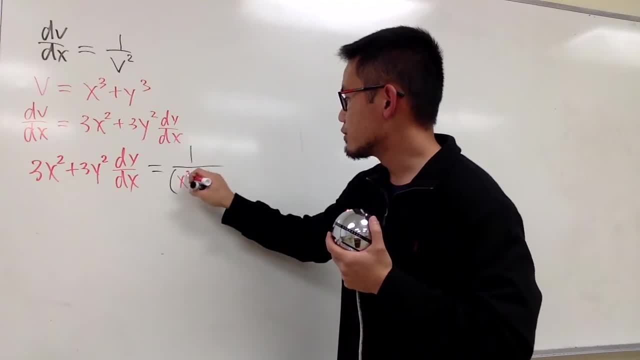 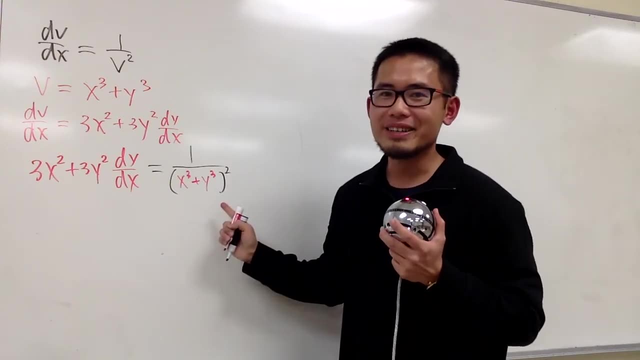 So I'm just going to open the parentheses and put this right here: x to the 3rd power plus y to the 3rd power and then square like this. As you can see, already right, This is now a much crazier looking differential equation. 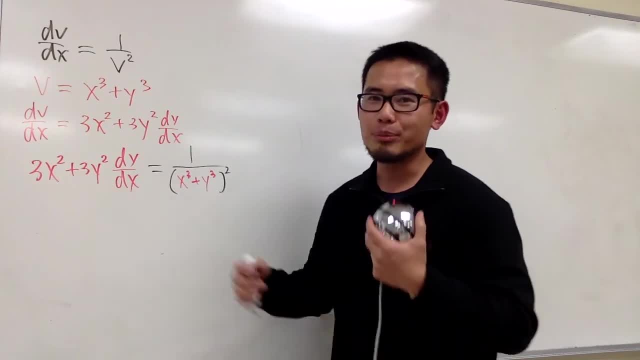 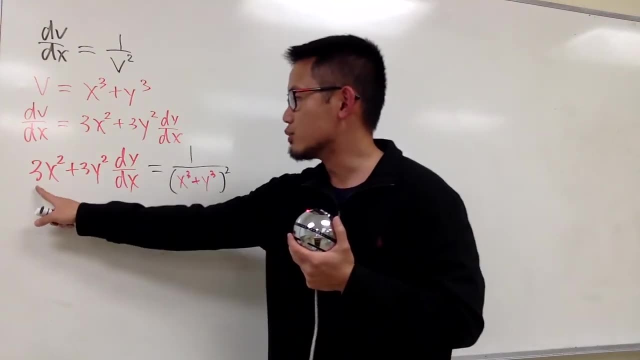 At the end I just had to isolate the dy dx and then I can present that to people and have them think about how to solve it, Things like that. Anyways, let me finish that for you guys first. So let me minus the 3x squared on both sides and you will have 3y squared dy dx. 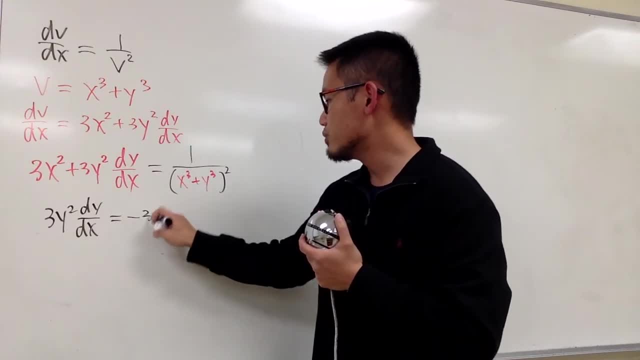 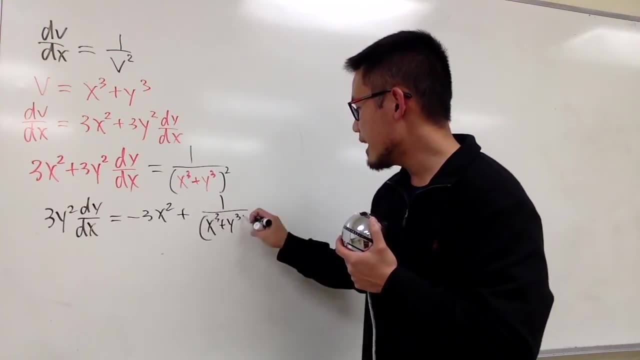 equal to this on the left-hand side. on the right-hand side it will be negative 3x squared plus that 1 over x to the 3rd power, plus y to the 3rd power, and then square right. 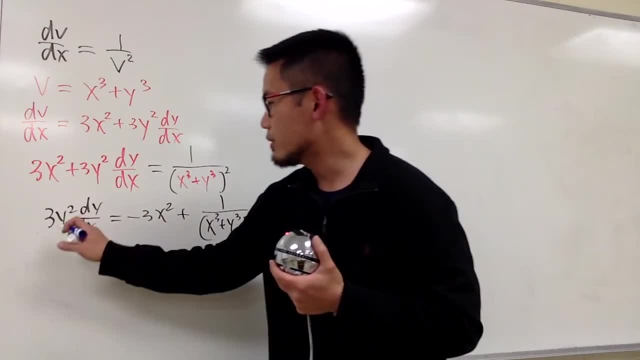 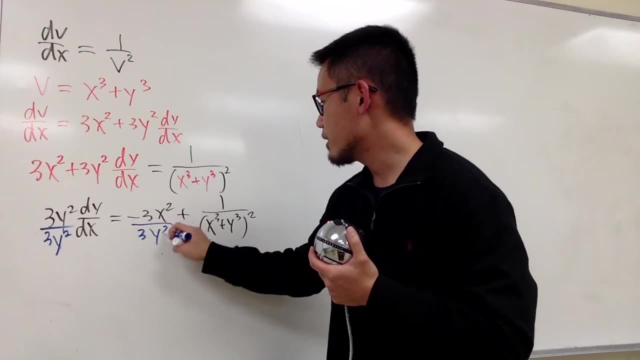 Well, I want to keep my dy dx clean, So let me just go ahead. divide everything by 3y squared y square, and this is my y, and then divide this by 3y square and divide this by 3y square. 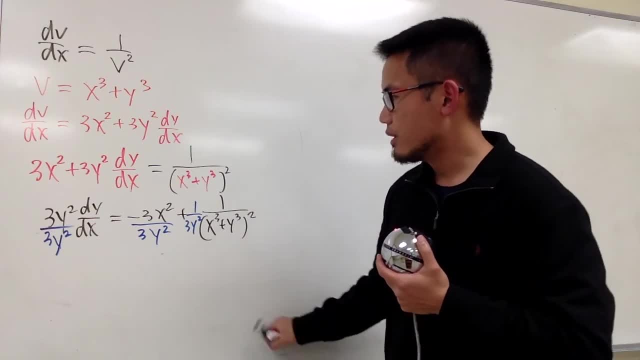 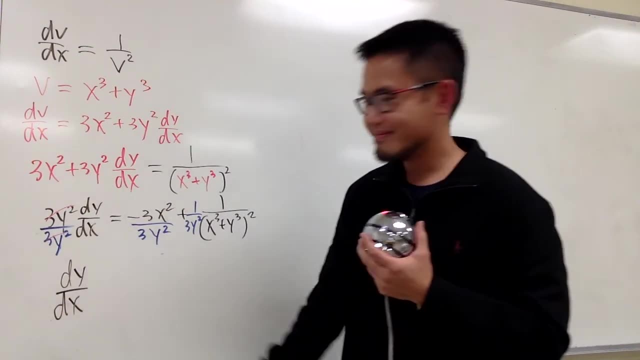 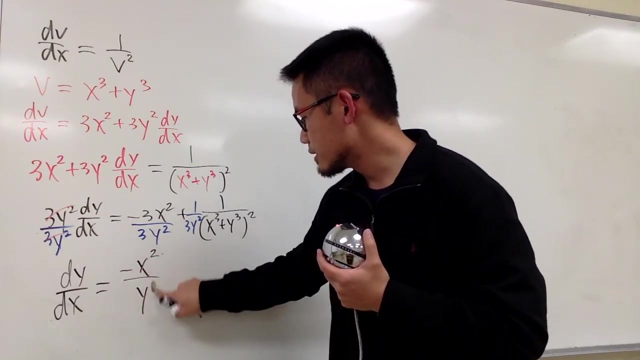 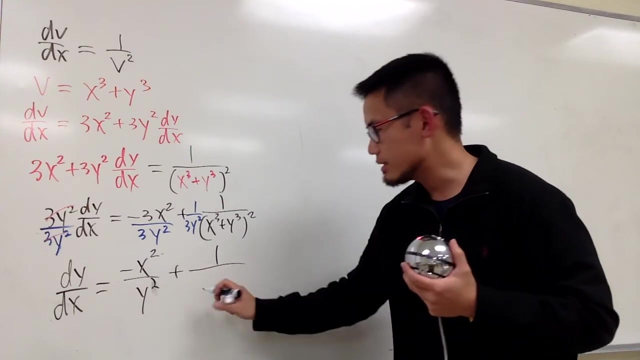 so let's put it down like that, and you see that this and that will cancel, we will have dy dx, this will be 3 and 3 cancel. so we have negative x square over y square- this is my square- and we add it with 1 on the top right, 1 times 1, and then we have this: 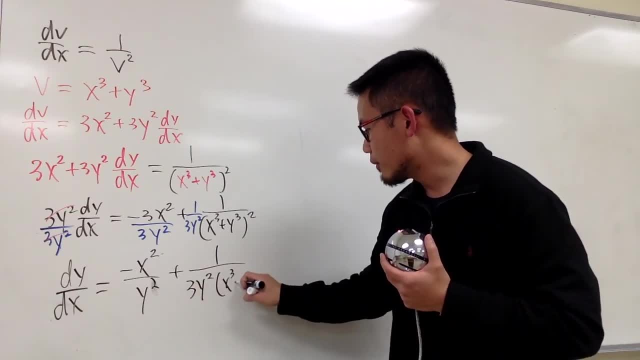 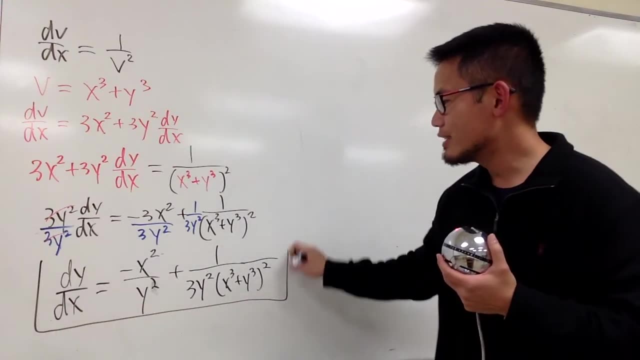 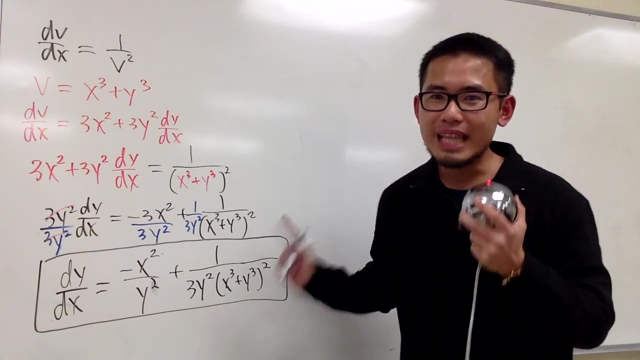 3y square times x to the 3rd power plus y to the 3rd power, and then square, and, ladies and gentlemen, this right here is a very crazy looking differential equation, and the way to solve it is to let v equals to x to the 3rd power plus y to the 3rd power. 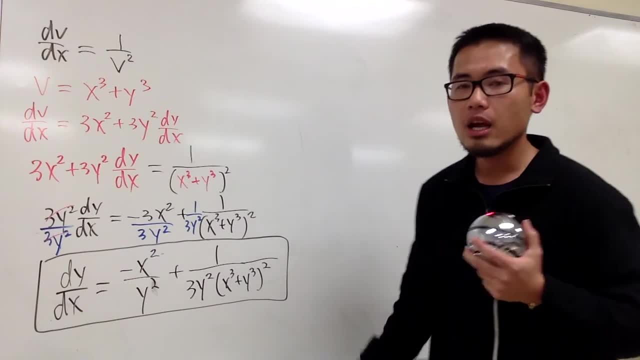 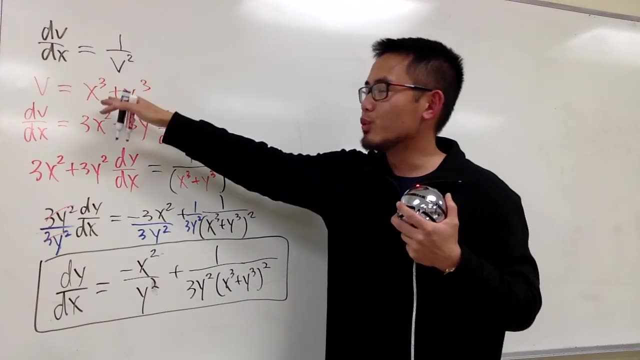 Because we decided to be like this. and, of course, once again, you can start with any easy differential equation right in terms of v, and then let v equal to whatever x and whatever y together and you can create your own differential equation that you will be. 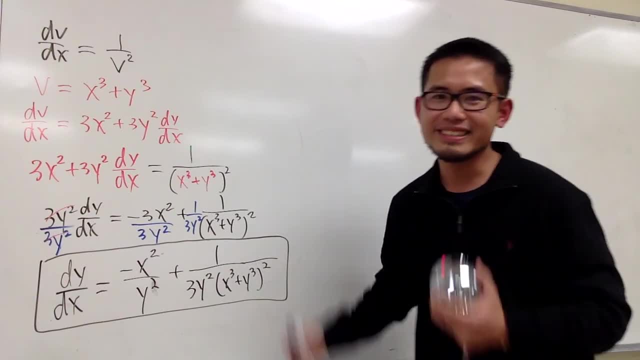 the person who knows what a substitution is. That's it.